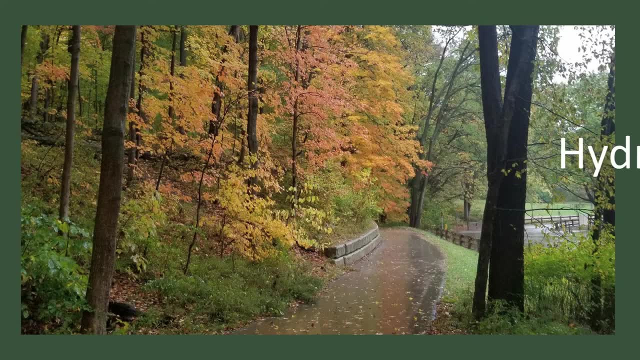 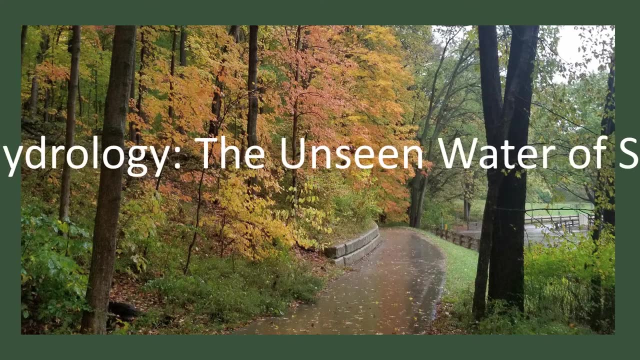 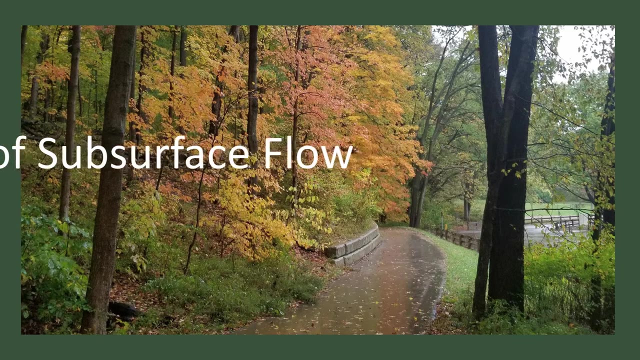 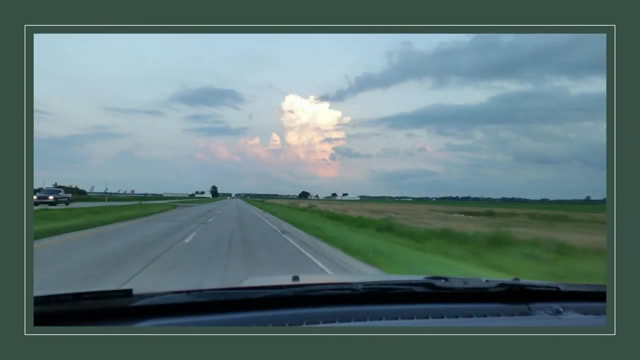 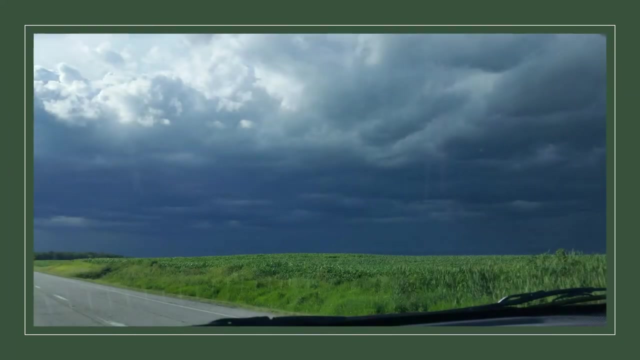 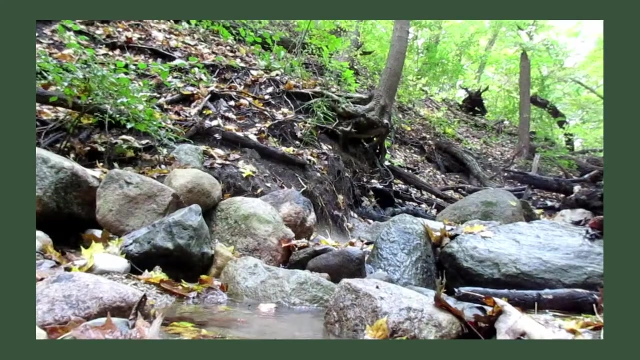 Hello and welcome to today's talk on hydrology, the unseen water of subsurface flow. Subsurface flow in hydrology is all of the water that the ground is able to absorb from precipitation and then moves either through gravity or evaporation. We're going to talk. 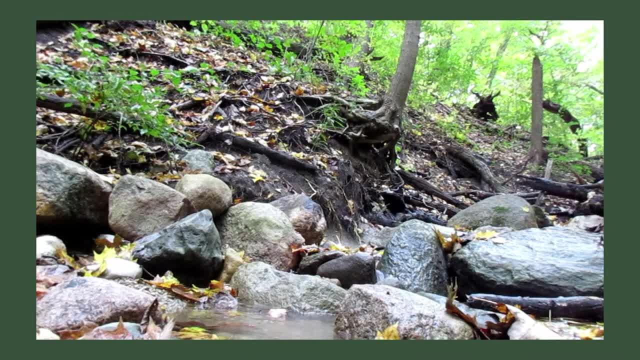 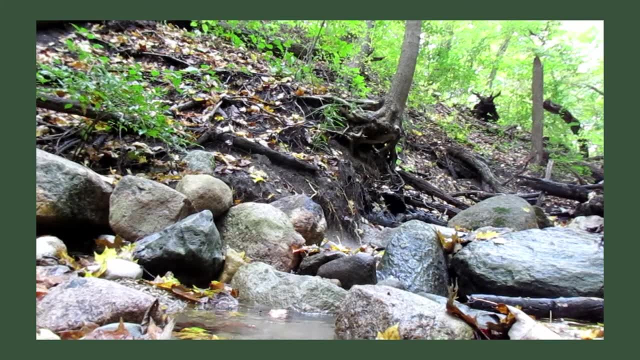 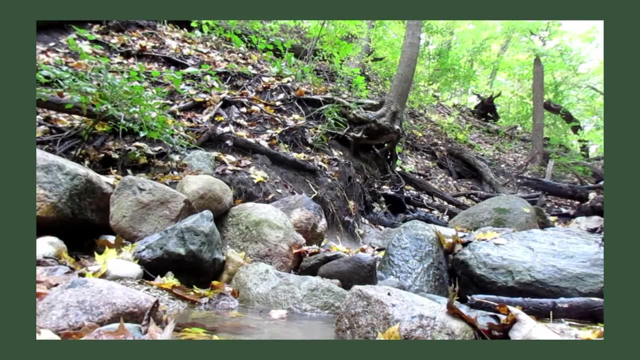 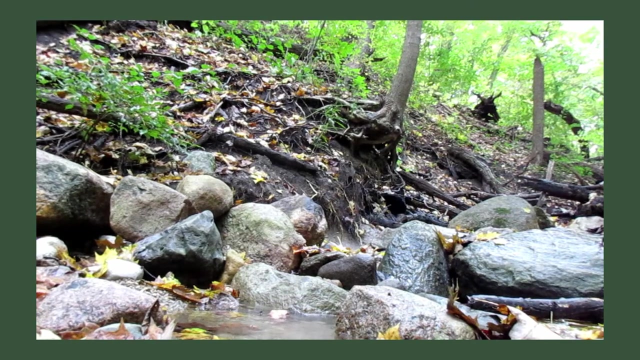 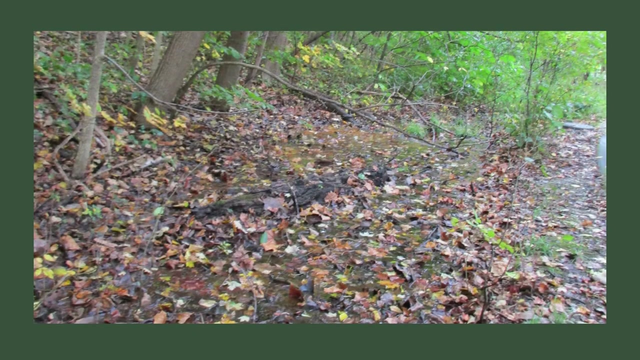 about saturated subsurface flow, losing streams flow and piping flow today, and how each of these components are affected by the environment that they exist in. The first mechanism we're going to talk about is saturated subsurface flow. Saturated subsurface flow is usually found in: 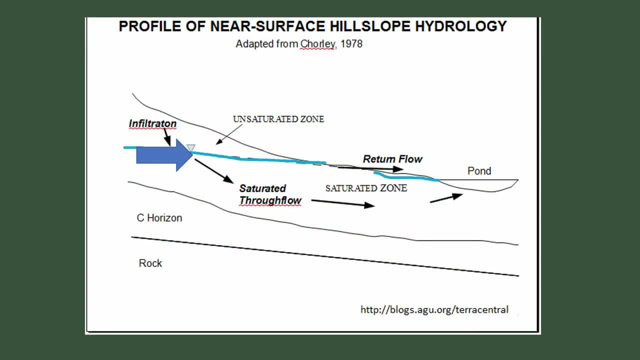 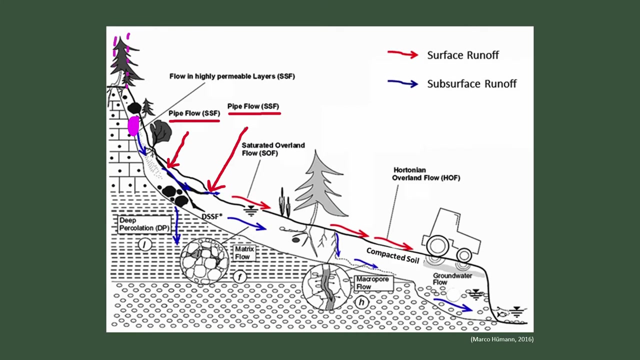 hills, slopes, back slopes and relatively flat places. The ground becomes saturated and the water seeps to the surface but continues to flow downstream. The next mechanism we're going to talk about is piping flow. Much like the naming implies, water begins to move very quickly through the subsurface as water. 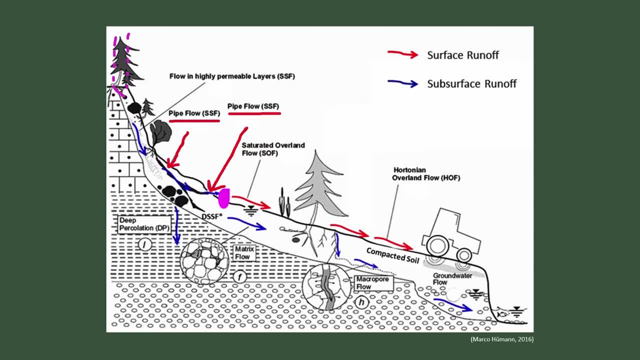 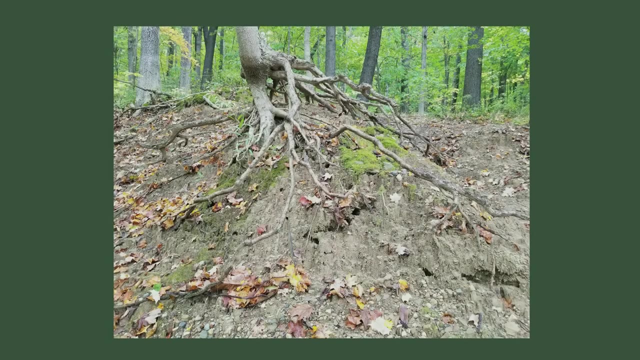 through pipes and then emerges at some sort of break in the soil surface. Most of the time, this break is either through a mechanical or a natural erosion cut into the topography of the land. Sometimes the holes are very small and other times they're very large. 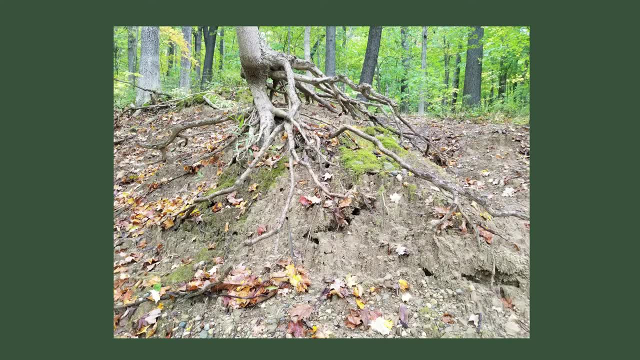 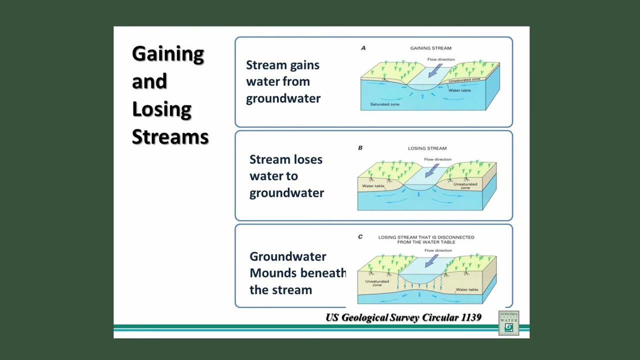 Streams are usually gaining or losing, and sometimes losing. streams are completely disconnected from the water table. These streams are usually classified as an ephemeral and they're dry most times of the year. Happy Hollow Park is one of those streams, as seen on the left, Only during.